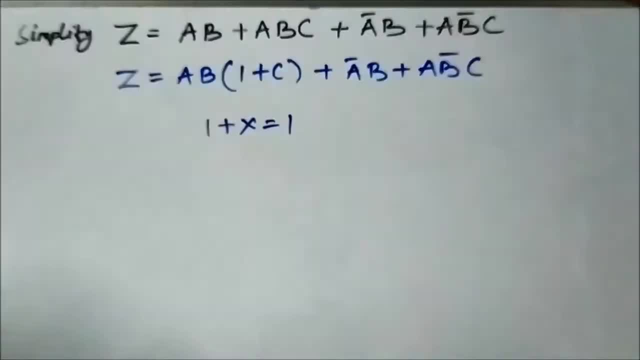 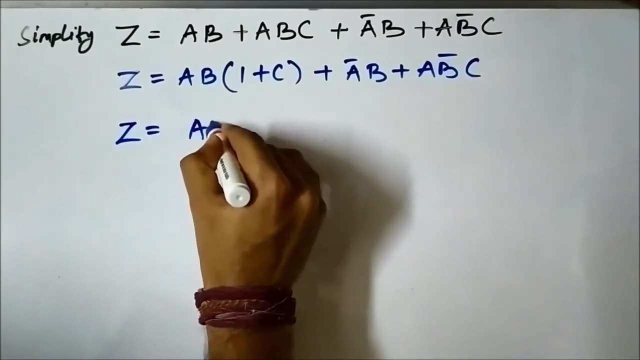 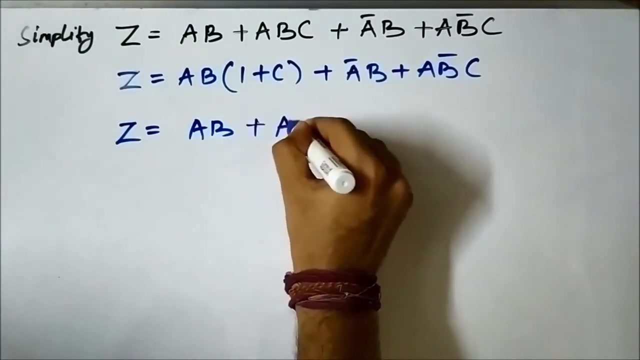 any Boolean variable. it gives us 1.. So 1 plus c will be 1.. So we can write it as z is equal to a b, simply because it will become 1 and a b into 1 will be a b plus a bar b. 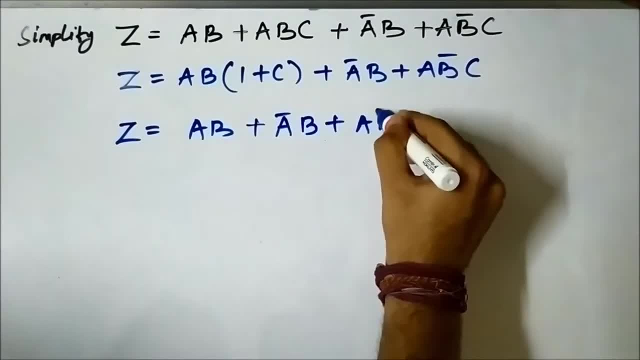 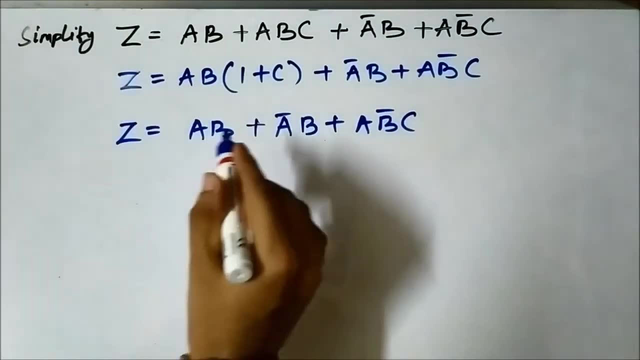 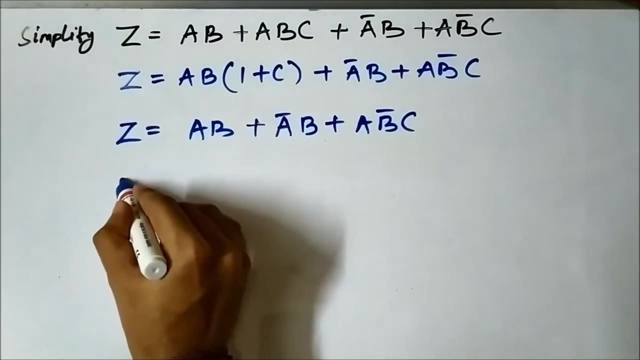 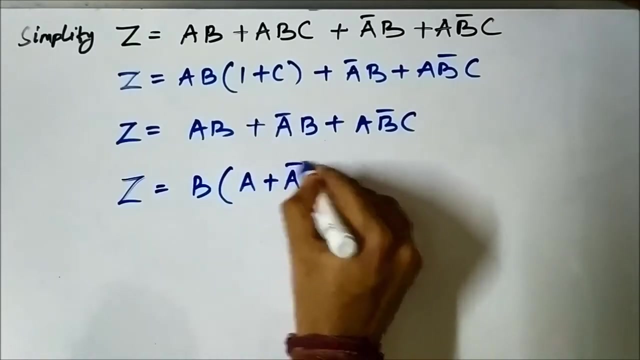 plus a, b, bar c. Again let us find out common terms or common variables. So here, in these two terms, the variable b is common, Here also there is b, here also there is b. So again b as common becomes a plus a bar, plus a, b, bar c. 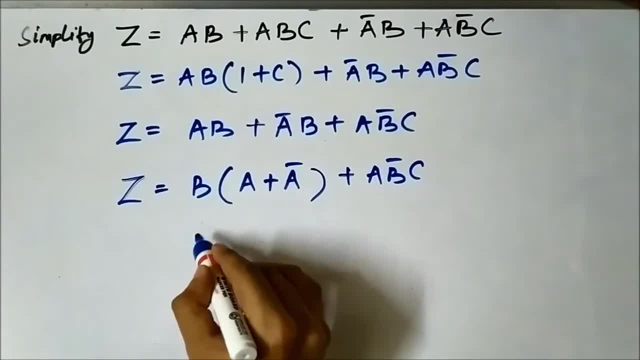 So here we can apply this Boolean algebra rule, which is any Boolean variable OR'd with its complemented version, gives us 1.. So a plus a bar will be 1.. So it is: z is equal to b plus a, a b bar c. So here we can. 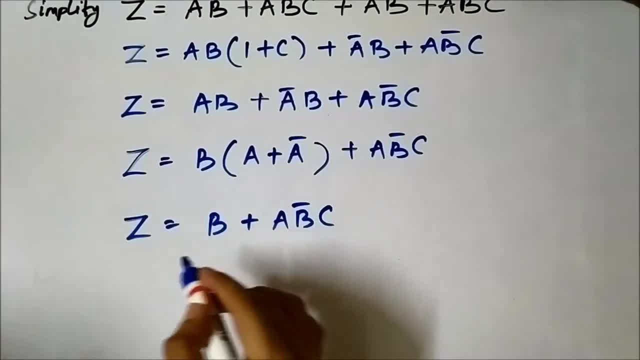 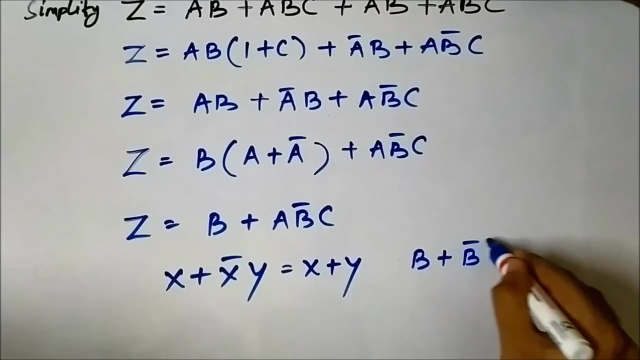 apply another Boolean algebra rule, which is the absorption rule rule, which states that x plus x bar y is equal to x plus y. So here this rule is applicable: b plus b bar into ac. We can rewrite it as b plus b bar into ac, ac combinedly taken as a single. 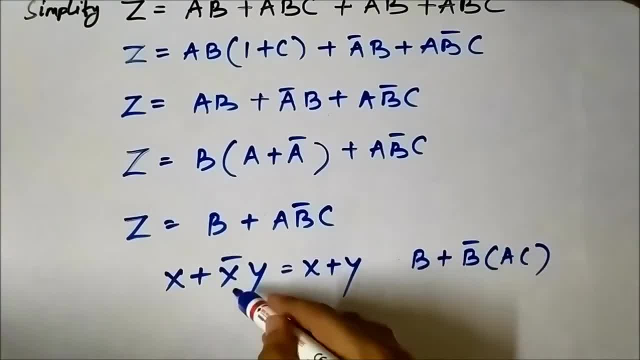 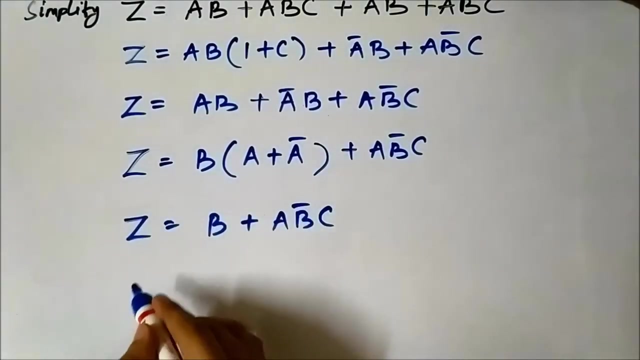 boolean variable y. So if we correlate these two, it is x plus x bar y, b plus b bar ac. x plus y will be b plus ac. So we apply this rule here and we get b plus ac. So here it is, z is equal to b plus ac. 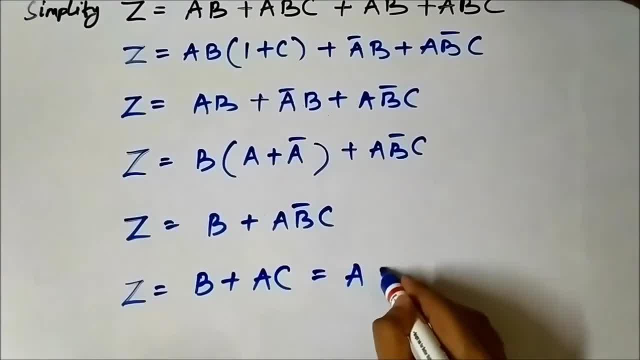 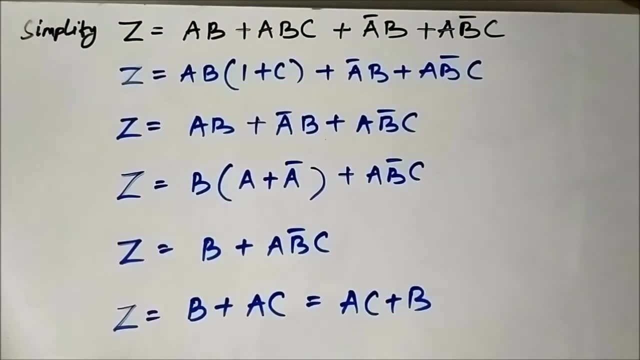 Or we can add it as ac plus b in alphabetical order. So there is no further simplification possible. So this boolean expression is simplified into this ac plus b. This is the final simplified boolean expression. So here is another boolean expression. 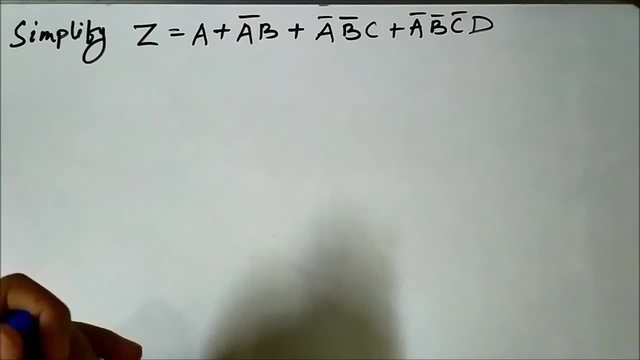 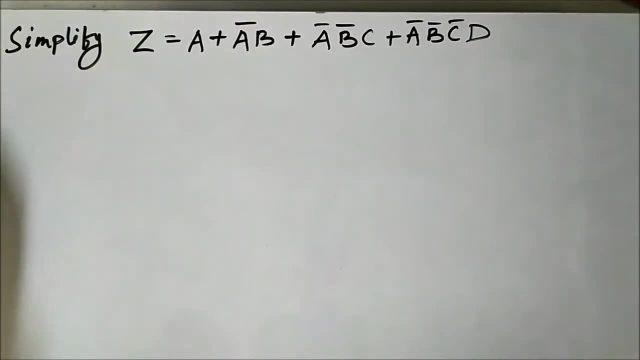 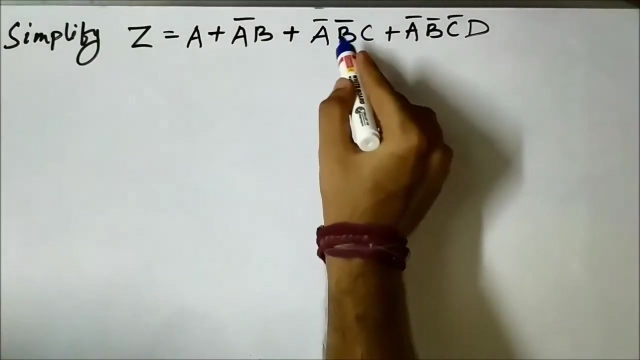 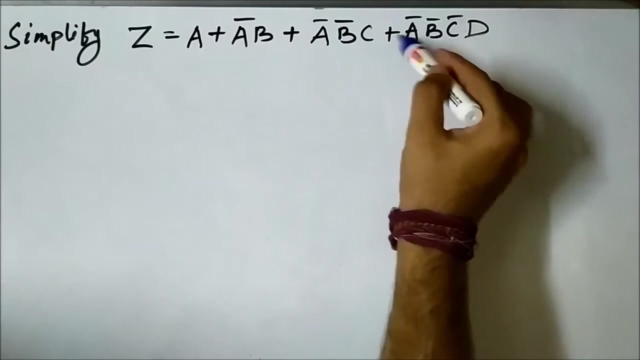 Which we have to simplify. So the first step again is to find out the common terms and then we will see how we can apply the boolean algebra rules. So here, if we look at these two terms, a bar b, bar c and a bar b, bar, c, bar d- Here a bar b bar is common in both the terms. 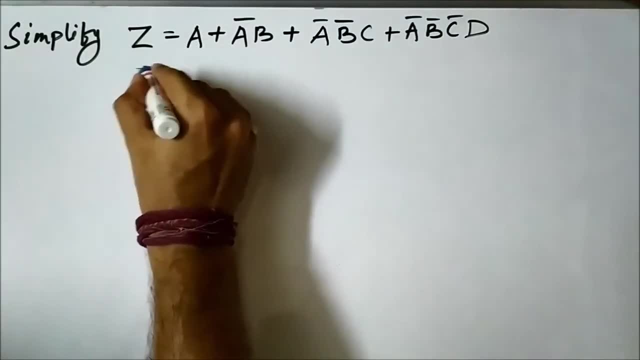 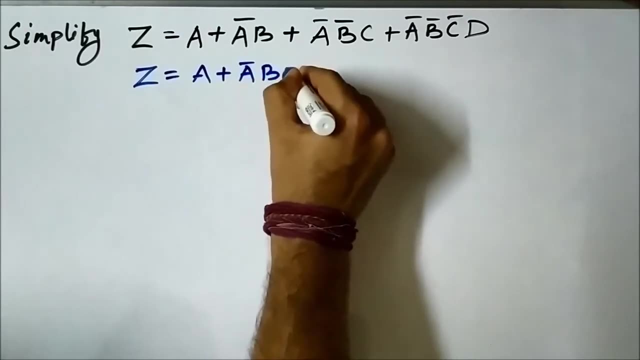 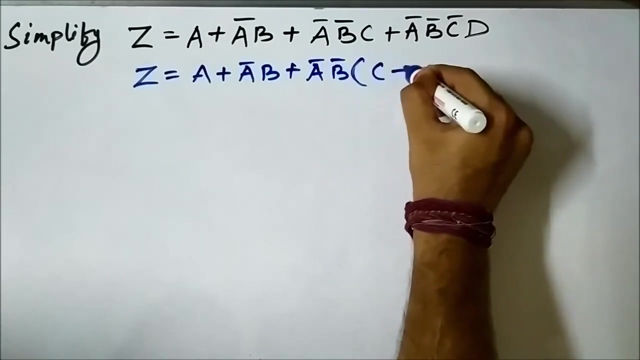 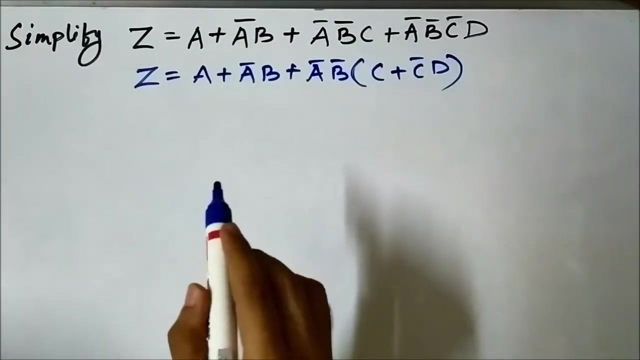 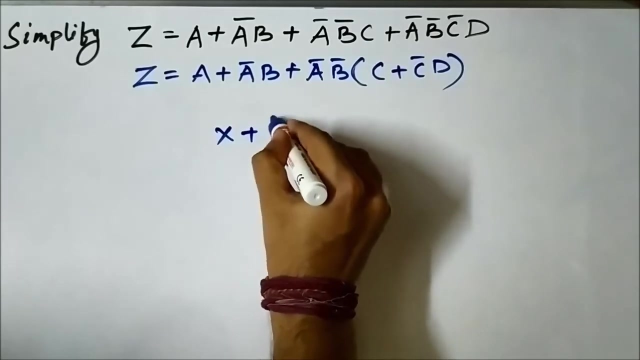 Okay, So let us take that as common. This a plus a bar b plus a bar b bar whole into c plus c bar d. So here we can apply a boolean algebra rule which is x plus x bar y is equal to x b bar, b bar c bar d. 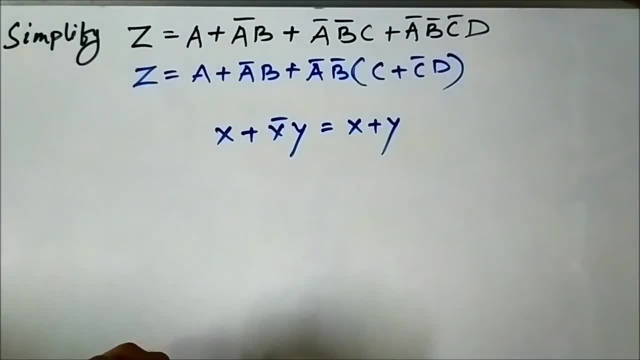 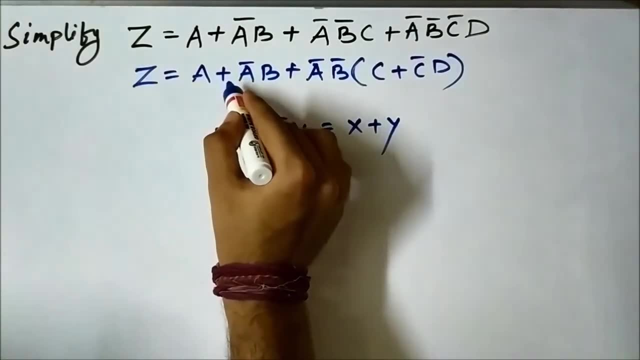 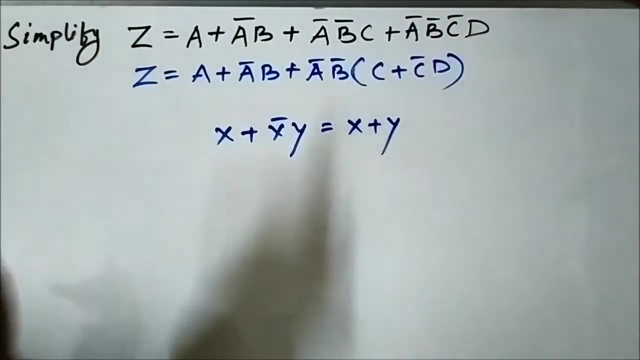 plus y. okay, we can apply that. actually, we can apply that here also: a plus a bar b and c plus c bar d. okay, so we'll apply it collectively: a plus a bar b will be a plus b, c plus c bar d will be c plus d. okay, let us apply this rule here in both the places. so it will be. 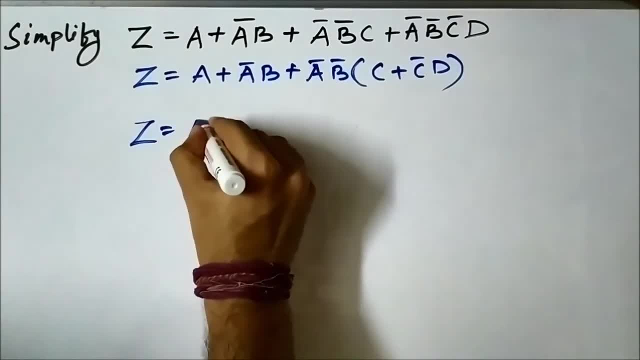 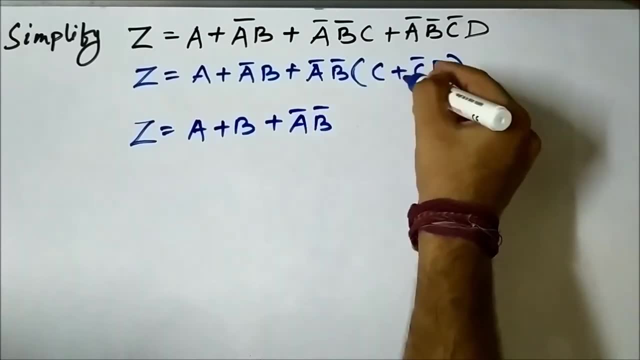 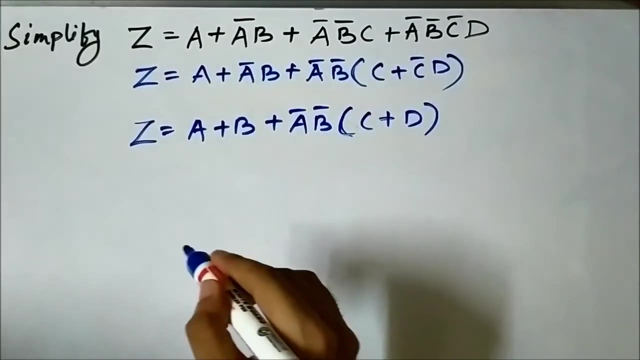 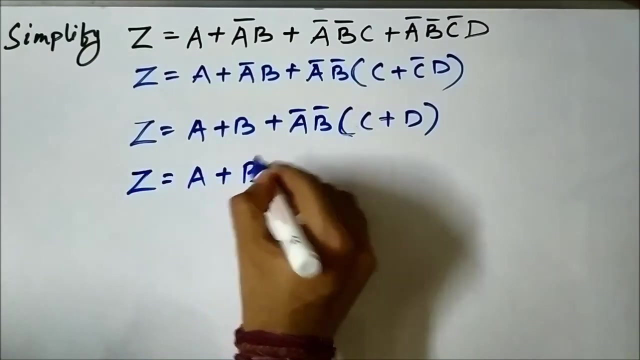 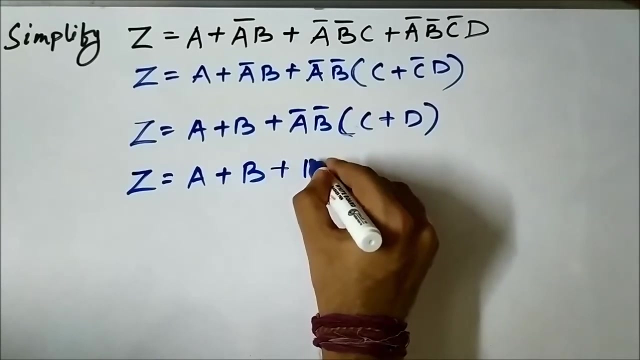 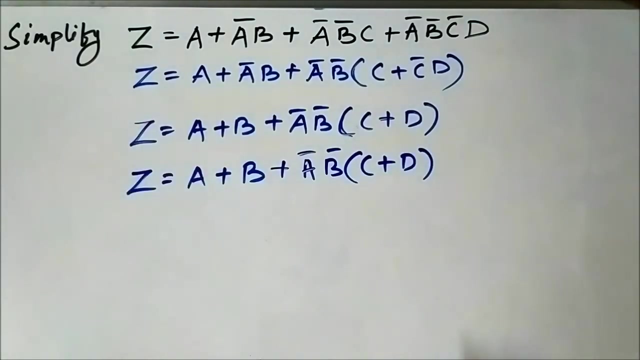 z is equal to a plus a bar b will be a plus b plus a bar b. bar c plus c. bar d will be c plus d. okay, so it will become: z is equal to a plus b plus b. a bar b bar you. we can write it as a plus b plus a bar b. bar to c plus d. So if we open up the bracket, 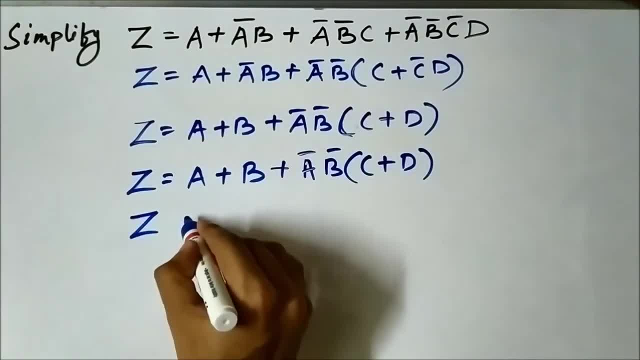 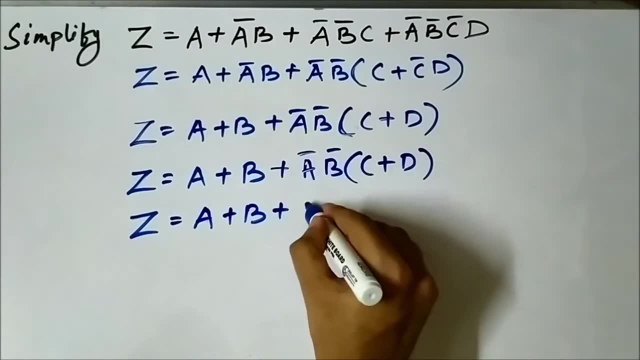 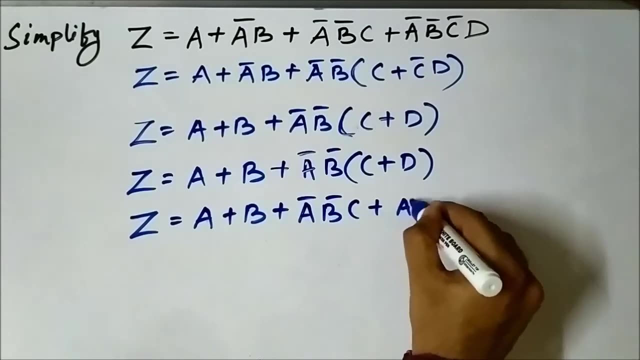 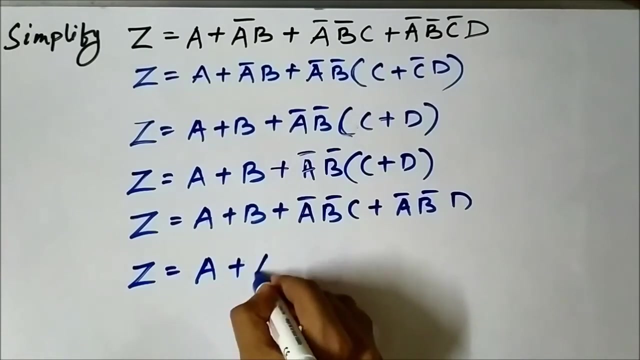 let us not open up. we will open up the bracket. then it will be a little bit easy. for us will be a plus b plus a bar b bar c plus a bar b bar d. Now let us split it. Let us write it as a plus a bar b bar c plus a bar b bar d. 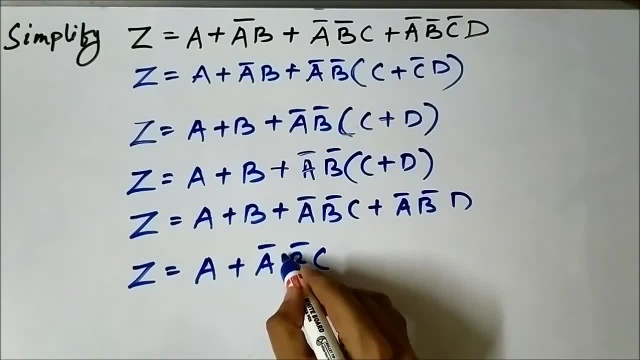 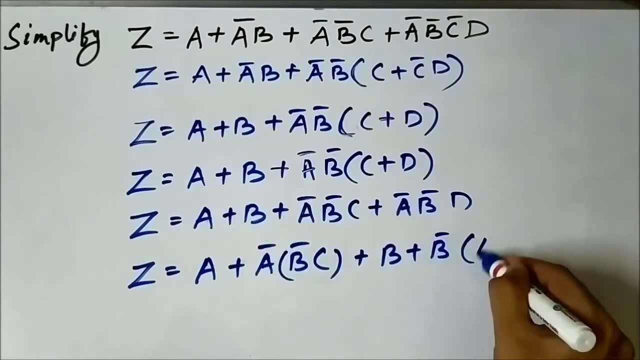 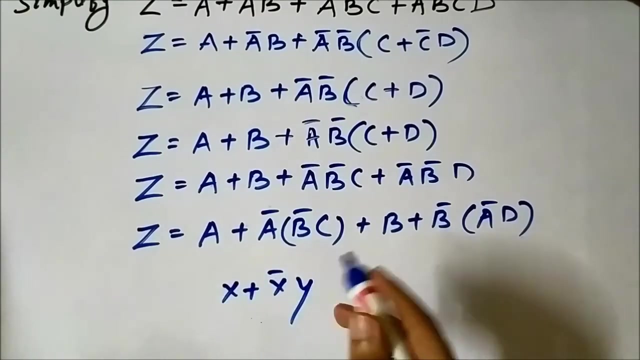 And here b plus b bar a bar d. this with this and this with this. So it will become. we can apply the rule: x plus x bar y is equal to x plus y. a plus a bar y. ok, bar this, taken whole, collectively it will become a plus b bar c. here it will become b plus a bar d. 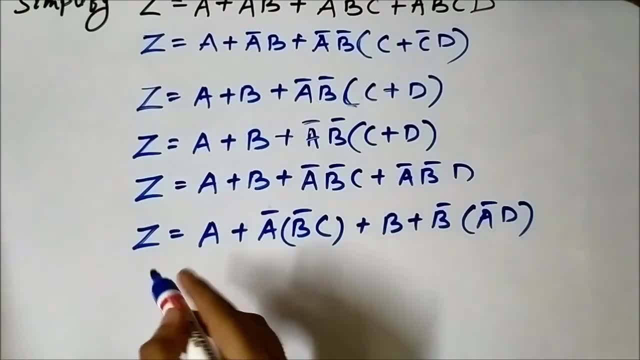 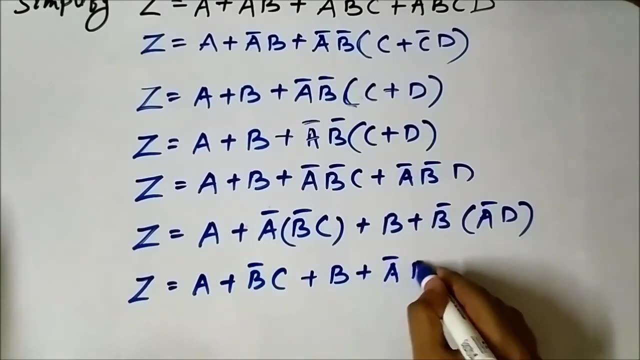 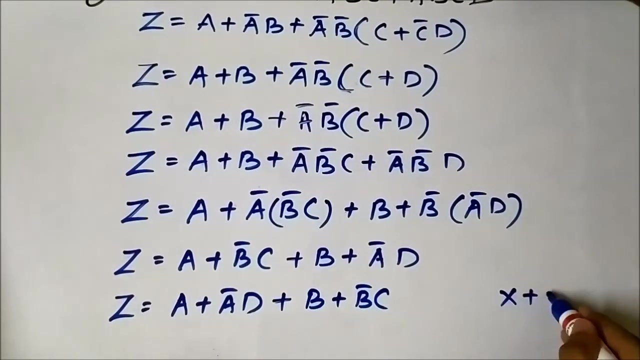 using this rule, So it will be: z is equal to a plus b bar c plus b plus a bar d. Now let us again arrange it in a proper way: a plus a bar d. we combine. we are combining this: a and a bar d plus b plus b bar c. again, we will apply the same rule, that is, x plus x bar y.